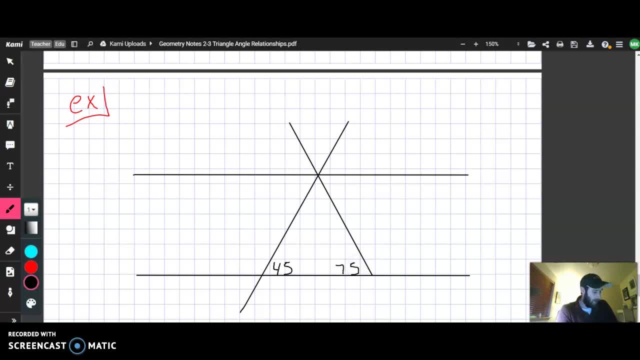 The other one down here is going to be 75. Based on that, our goal is to solve for x, x is to solve for y and we're going to try to solve for a and b. So our goal is to solve for x, y, a and b. The first thing we have to identify is our angle. 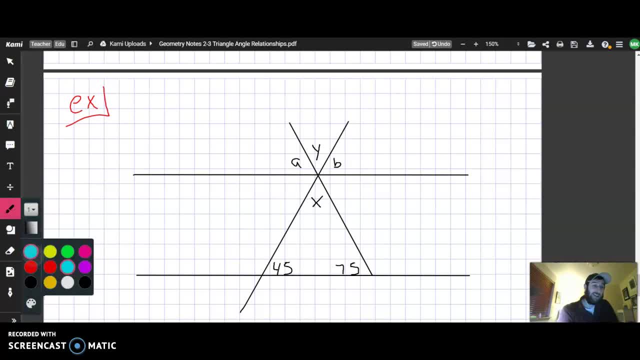 relationships. So let's go ahead and identify some colors so we can keep track of what we're comparing our angle relationships with to When I can look at a and b be. My first hunch is to identify the exterior angle theorem. The downside is: is that the 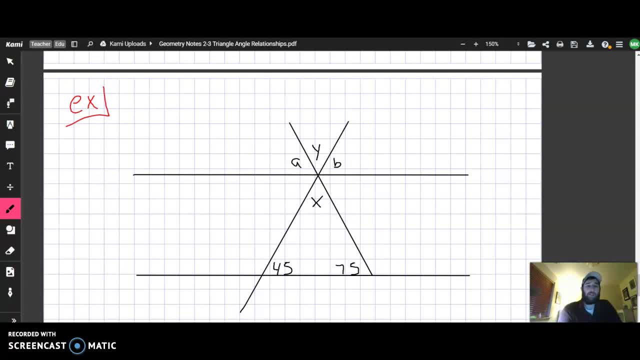 exterior angle theorem only works when it's the full angle, that's outside, And angle A isn't that full angle, It's only part of it. So the exterior angle theorem isn't what we're going to want to use. but we know that these two lines are parallel, And so if I compare this 75 degree measure with 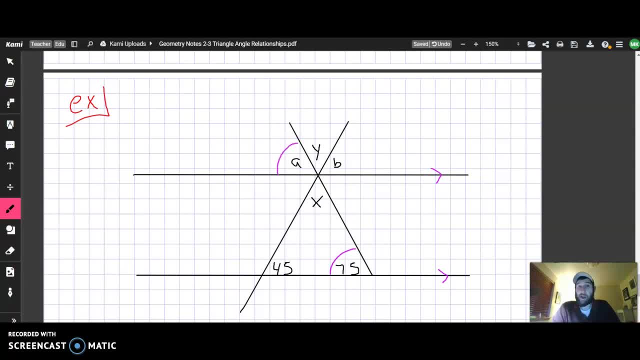 that angle A. well, they're matching. They're both in that top left hand corner And so A is corresponding with angle 75. And we already know that, know that corresponding angles are congruent. So our value of A is 75 degrees because 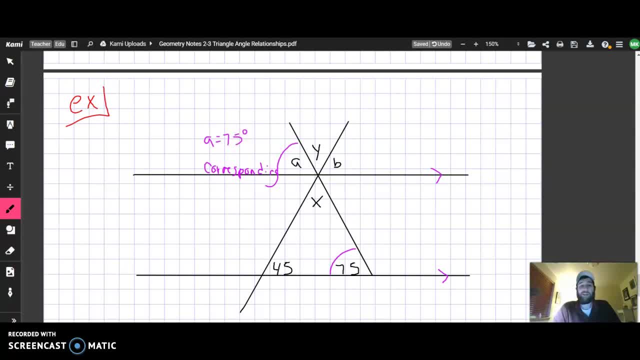 they're corresponding angles. Let's go ahead and take a look at angle B. You may already notice the pattern here that B and 45 also have that very similar relationship. They're both in that top right hand corner, so on those parallel lines B is also corresponding. 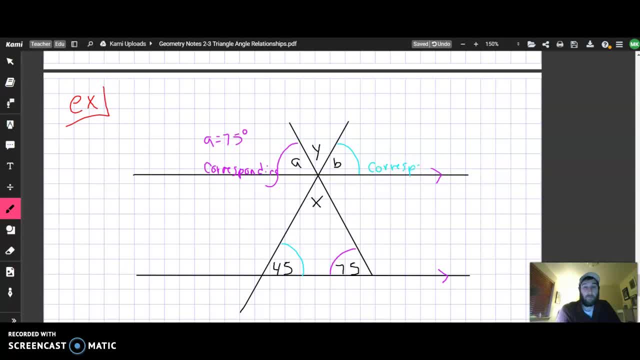 and because we know their corresponding angles. B is equal to 45 degrees, since corresponding angles are congruent. Now, those first two angles we were able to solve because we knew our angle relationships from our parallel lines Last week. Now for angle X. we're able to solve for angle X because we know our triangle sum.